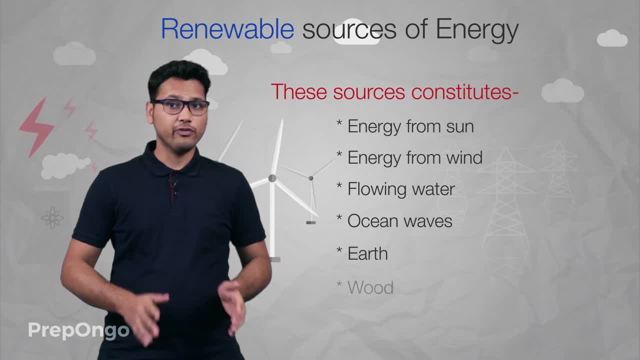 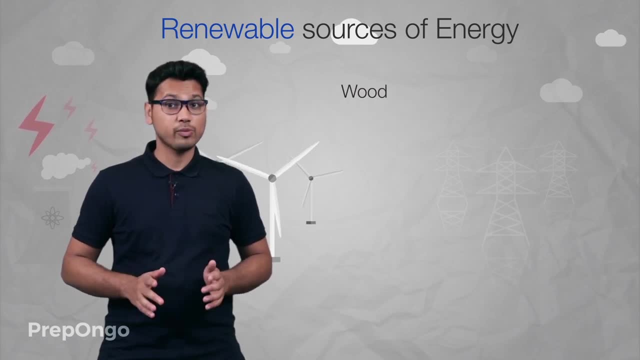 earth, etc. Now we can consider even wood as a source of renewable energy. But in considering wood as a renewable source, we have to plant the trees regularly and we have to take good care of them so that we can ensure that we are getting a continuous supply of firewood. 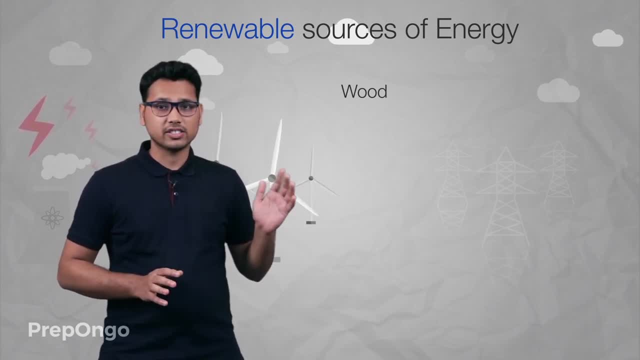 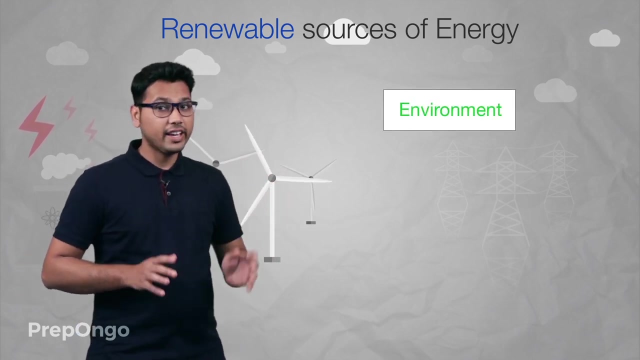 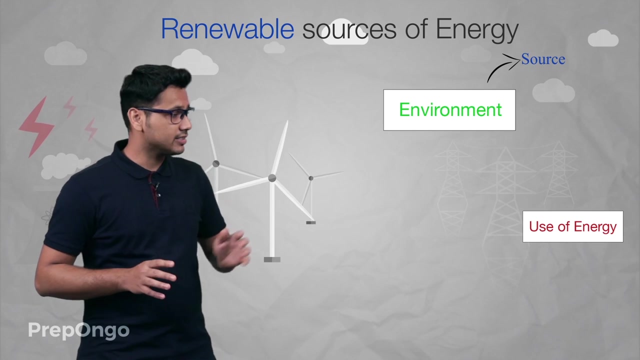 So we can consider wood as a source of renewable energy if we could plant trees on a regular basis. Now, if we try to understand the energy from renewable sources, let us consider this: We consider environment as the source here, and the energy from this environment is either used directly by us or it is either used indirectly. 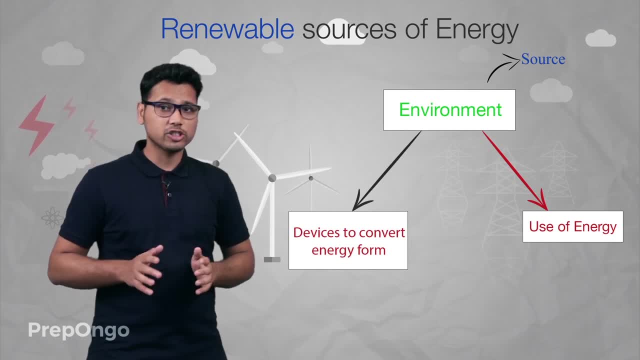 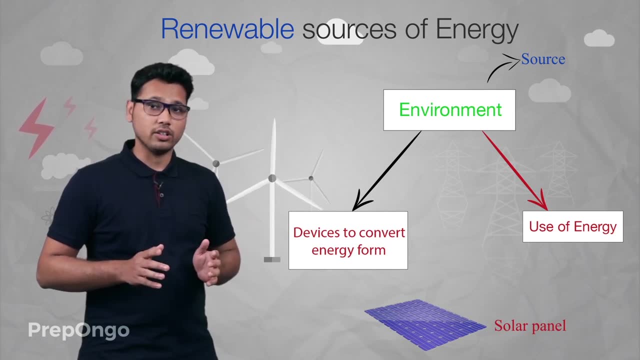 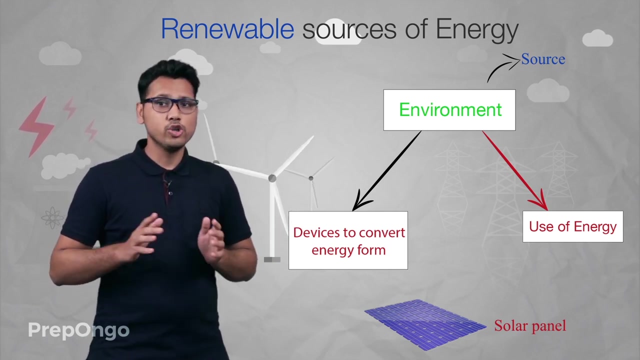 First it is being converted into some useful source of energy by using some device like solar panel, solar cells, which you will study later on. So it is first converted indirectly in some form so that we could utilize it, and then it is then transferred to some 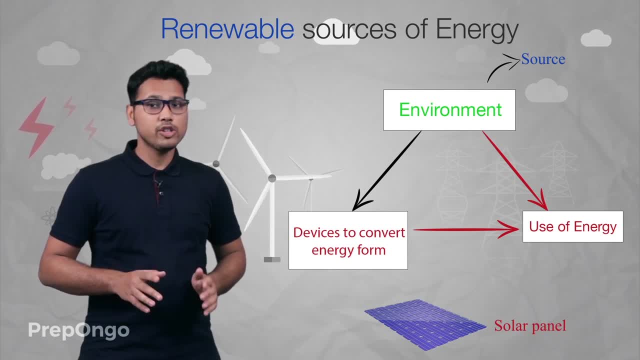 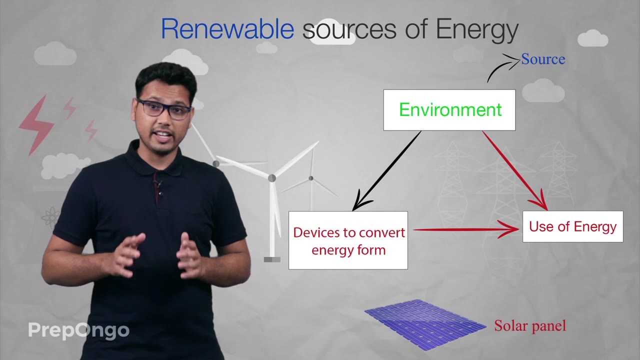 usable form. by using this device. Now you may find out that, since energy is directly coming from the environment, so we can say that till the environment is there, like sun or wind or ocean are there, we will be getting this type of energy, So we can say that renewable sources are non-lasting sources. Now let 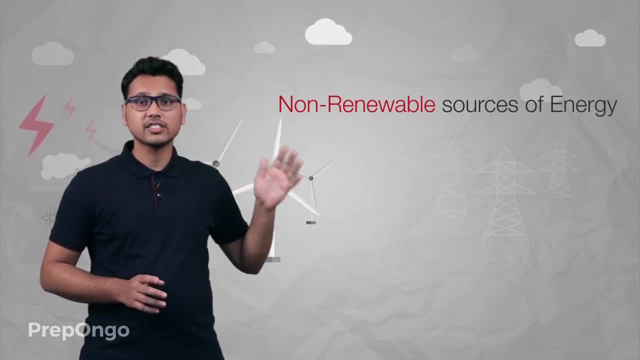 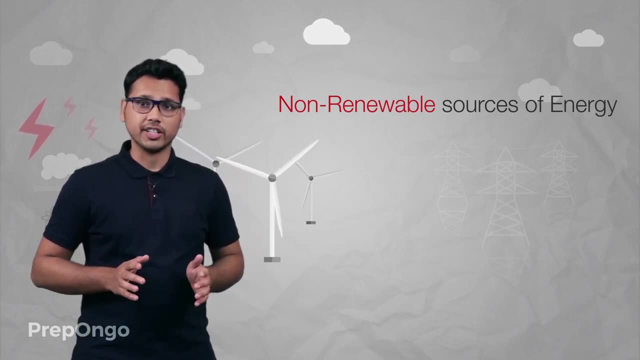 us have a look on the second sources of energy, which is non-renewable sources of energy. now, as the name suggest, these are the sources which cannot be regenerated, or we can say that the reserve is limited and hence they are also called about that these energy resources with discussed above The second source of energy which cannot be regenerated, or we can see that the reserve is limited And hence they are also called. 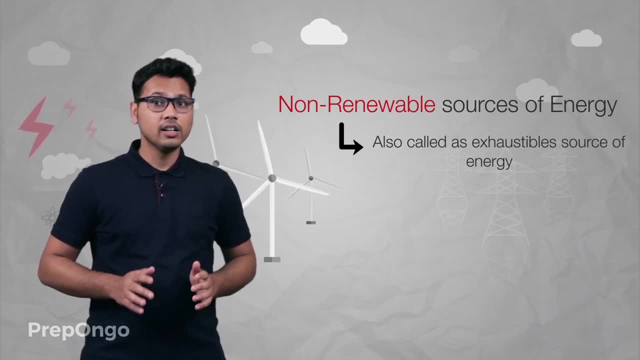 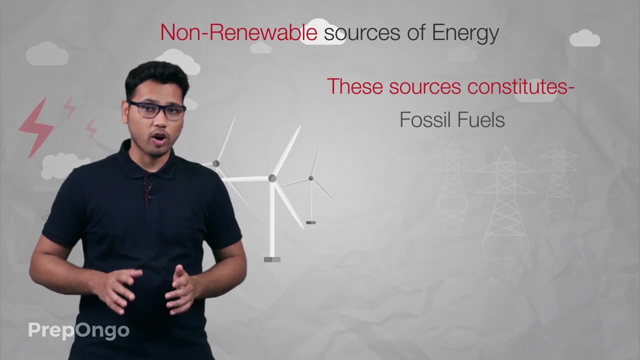 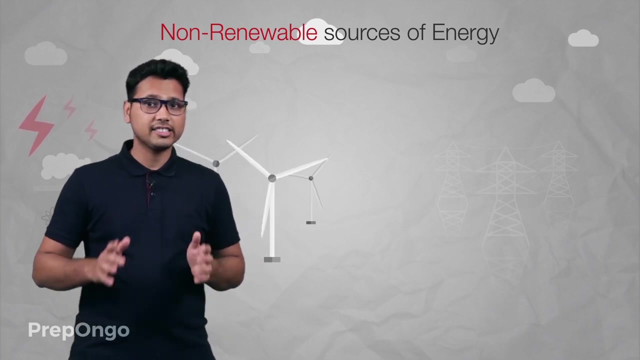 exhaustible sources of energy, as once they are used, they cannot be made again. Now these sources constitute energy from the fossil fuels like coal, petroleum and natural gas. Now let us look at the utilization of energy from the non-renewable sources. Now, unlike renewable sources, we cannot use energy.